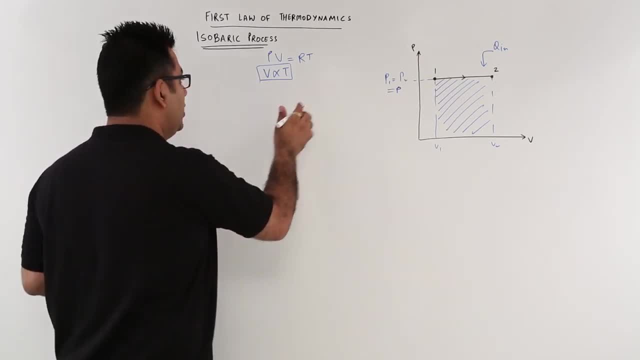 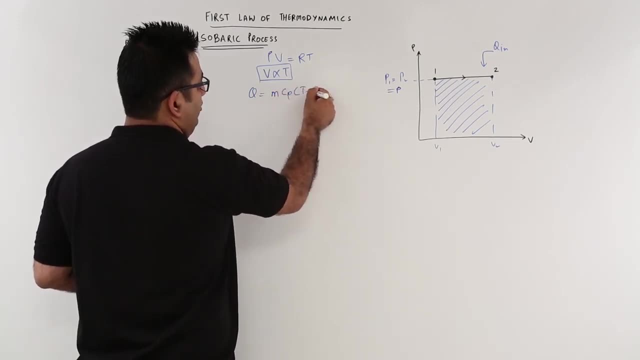 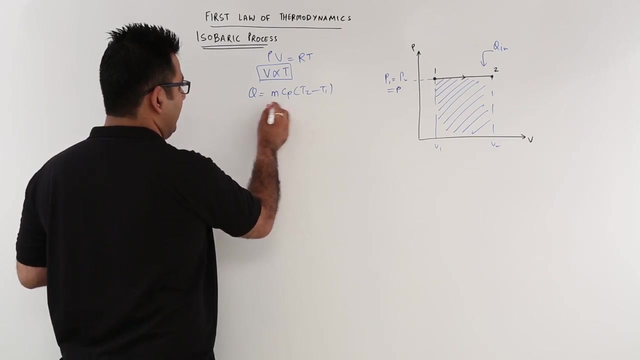 from that gas at constant pressure. Now, whatever heat interaction that you have, you will have one form of crystal charge that you have. So this is the case of T2.. So these are the четы abovefs. So this would also be the stress места. 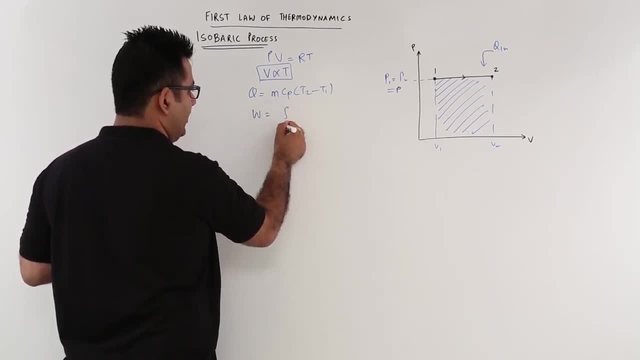 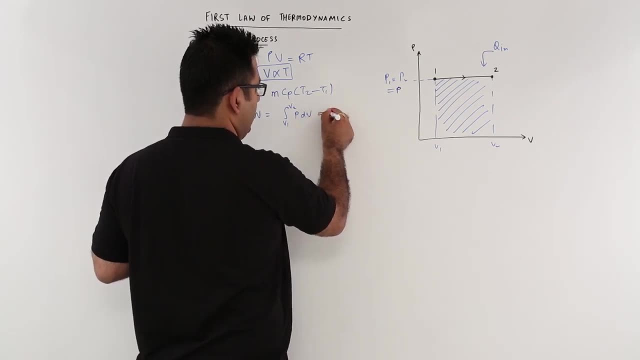 software. this is theegerdal formula, So this is the paper flip. this is the paper flip, So this is a proof, or liquid soluble. So with this surface you would decrease the temperature. In the example that you have, it can be found out by M into C, p into T, 2 minus. T 1, simple I can say a formula for heat cultivation. If you have to find out the work done, that is integral V1 to V2 into PdV. that is the formula. So if you look at, this is equal. 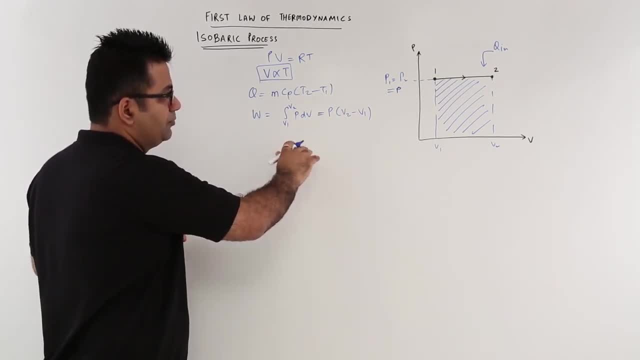 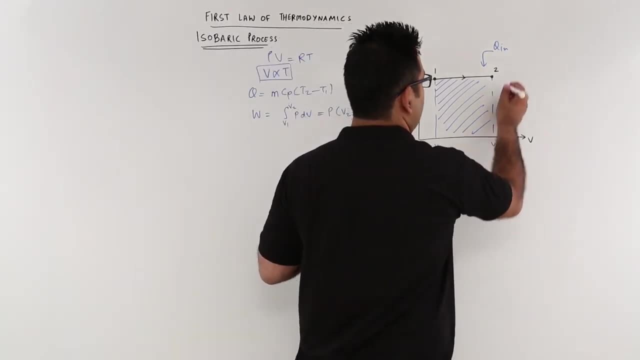 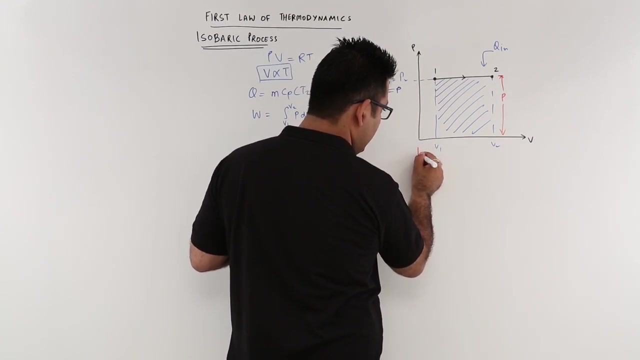 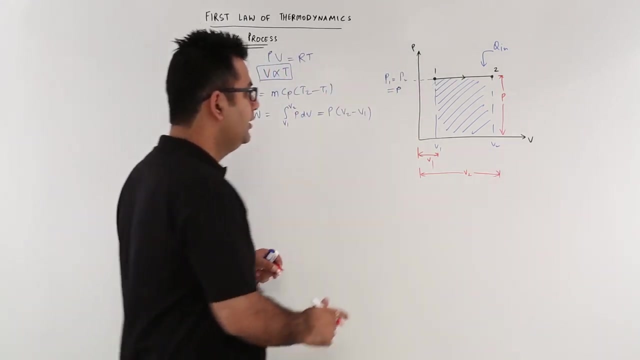 to V2-V1.. Simple, OK, 웠ardi Quốc trịnh ỷ huி有點 corts ra wreckure that corresponds to the area below that curve. because if you look at this, this length, this is P pressure value, this is V1, this is V2, I need the length of this dimension. 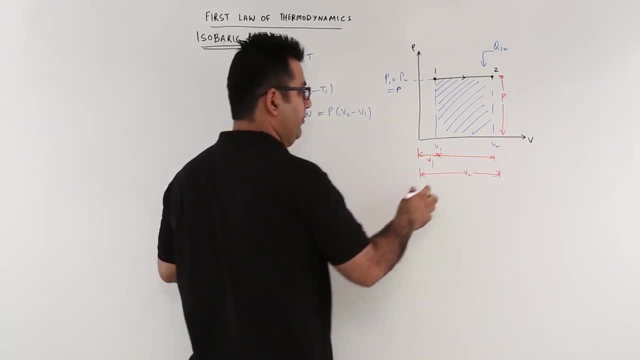 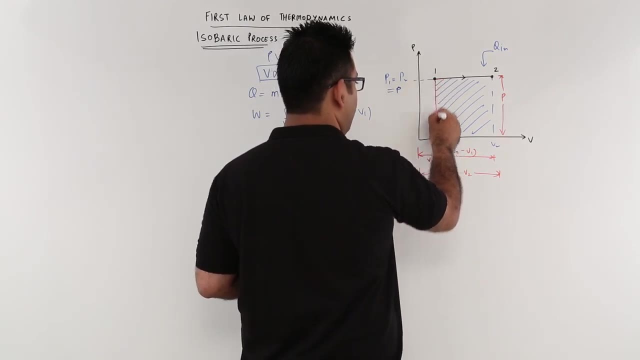 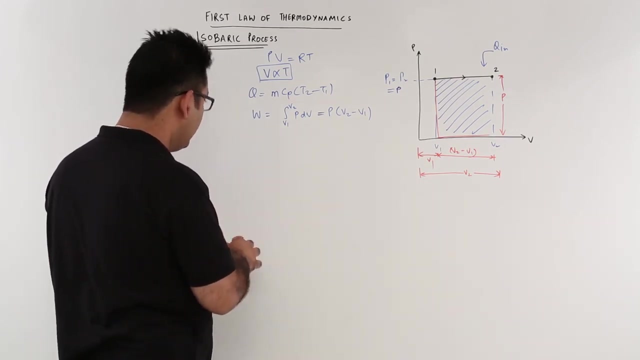 that is V2-V1,, so that would be V2-V1,. so the area of this rectangle would be this: into this, that is P, into V2-V1, this one, okay now the value of change in the internal energy. 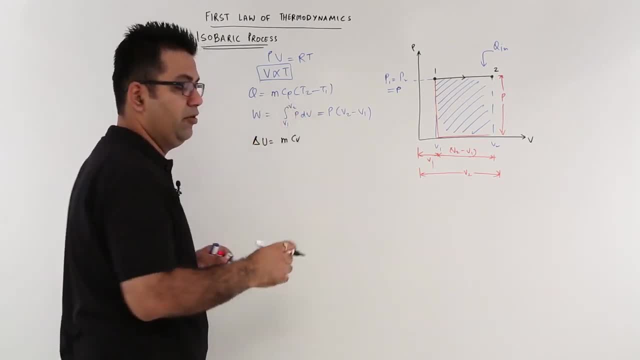 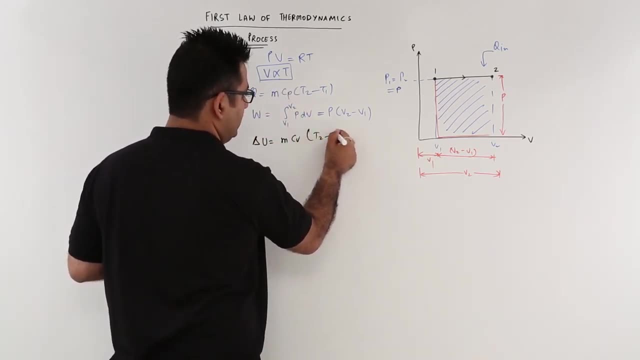 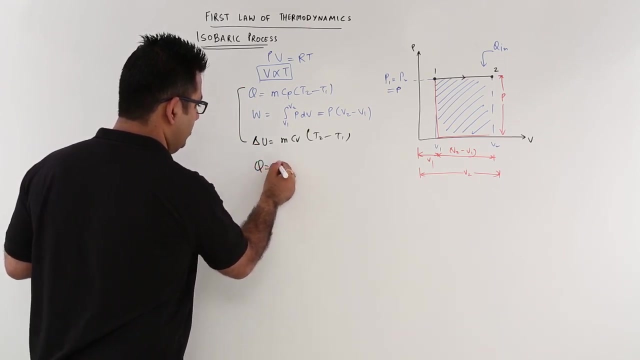 that is delta. U is equal to M into CV. now U always has CV with it. it does not have CP, understood? That is T2-T1,. now simply apply the first law. so you have: Q is equal to W plus delta. 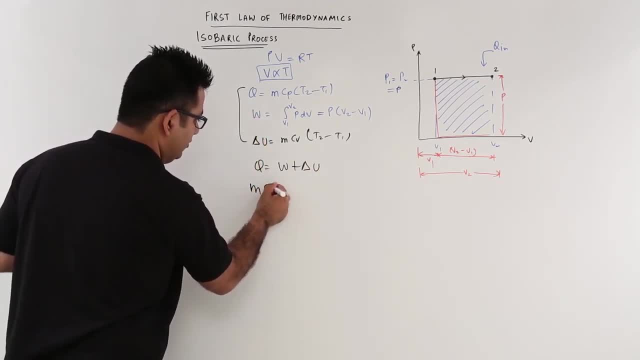 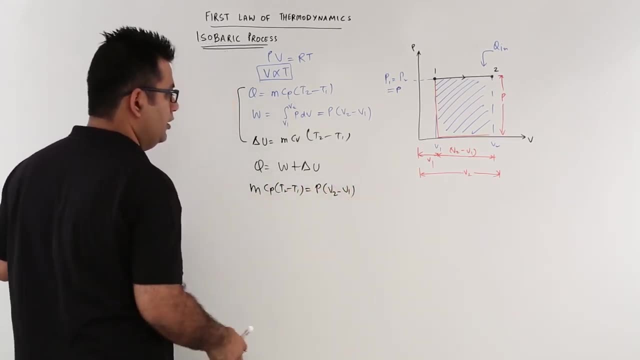 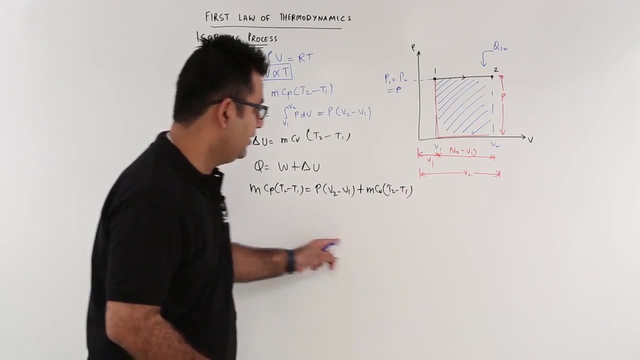 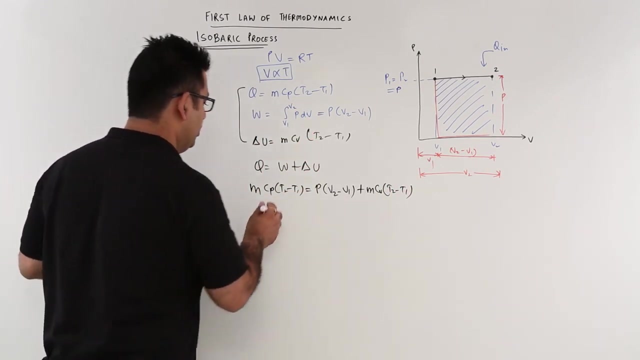 U. so this becomes M into CP into T2-T1, is equal to pressure into V2-V1 plus M into CV into T2-T1, so this is the mathematical relation For the isobaric process and the application of first law on this process. so this is Q.